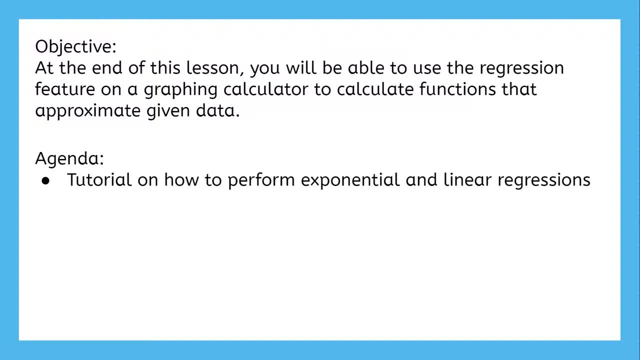 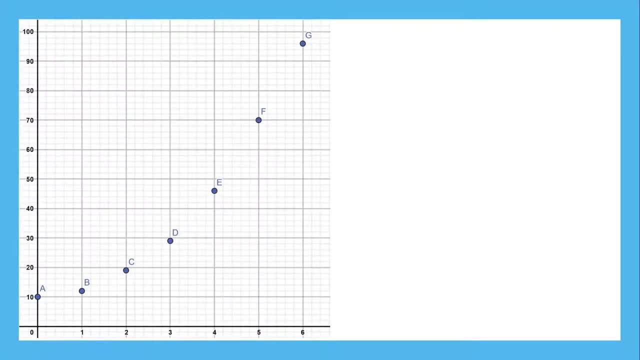 tutorial on how to perform both exponential and linear regressions, and then you'll have a chance to try it yourself with a practice example. We can agree that this graphed data set has a distinctly exponential shape, right Cool? So let's find the function. The initial value is 10,. 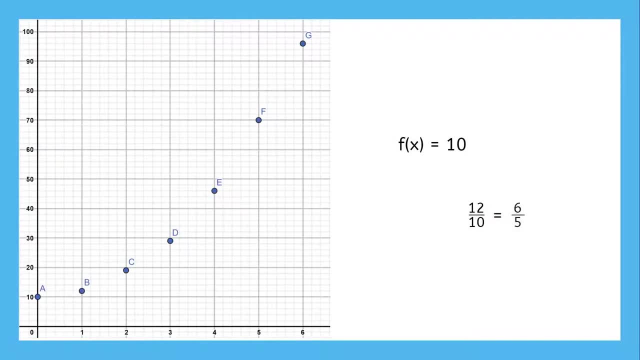 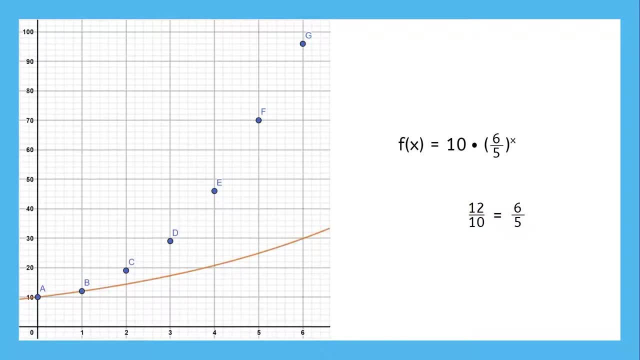 to the x power, which looks like: uh, this? Well, that's not right. It doesn't go through all the points, But if we change that initial value it won't go through point A anymore, and if we alter the growth factor it'll grow at a different speed and it won't pass through. 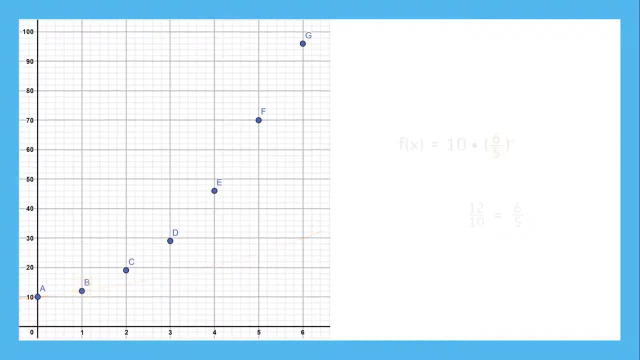 point B. The problem here is that we assumed these points were on a perfect exponential curve with a definite function, rather than the data being approximately exponential. There actually isn't a function that will pass through all of these points, But we can use technology to create a function that approximates the data as perfectly as possible using a. 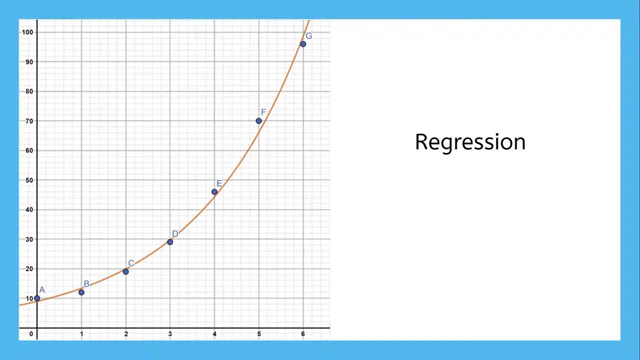 technique called regression. There are all different types of regression and since we use it to approximate data with an exponential growth function, this would be called exponential growth regression. Most graphing calculators have the capability to do some forms of regression, but each calculator is different. 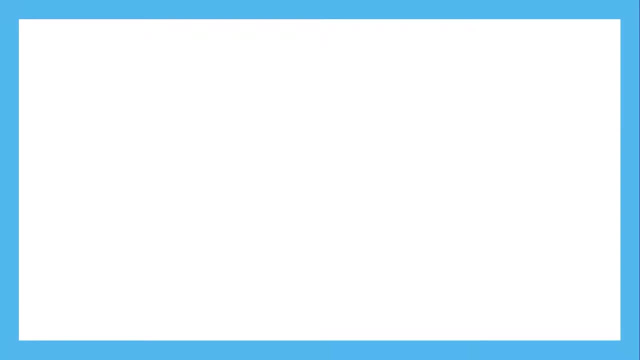 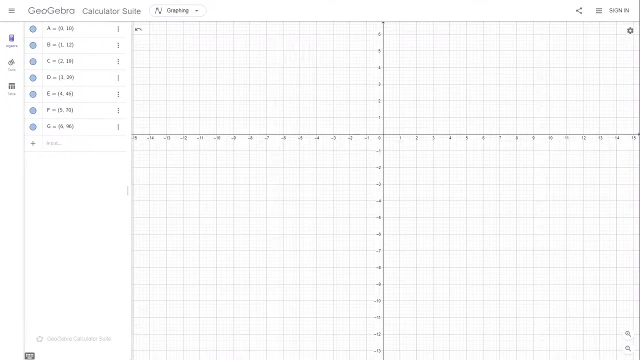 So, for the sake of this demonstration, we'll be using a graphing calculator that everybody has access to. Interactive, free online graphing calculator from Giogebra. Take a moment to open this website in another tab. Here's the data from our first example. Pause the video while you type this data in on your 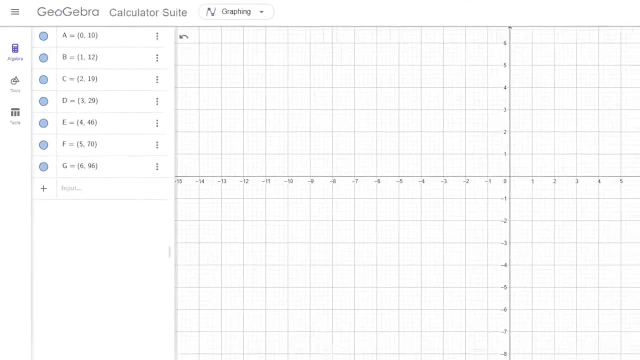 own screen. The points you entered have already been graphed. We're just too zoomed in here, But you don't have to read through them again. We'll just zoomed in to see them. so let's change the viewing window. 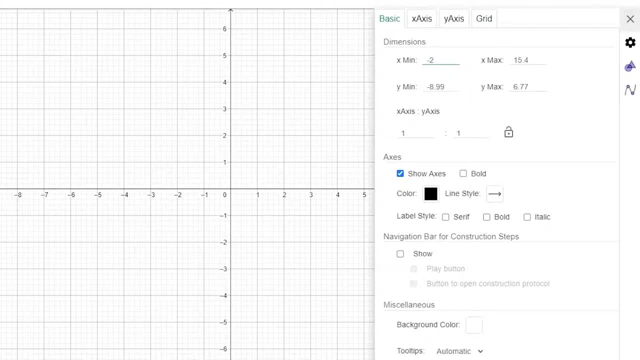 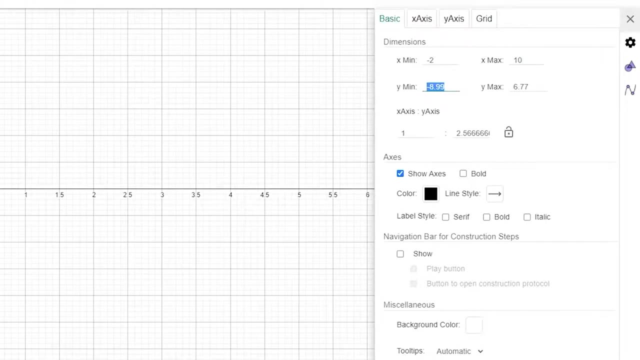 Our x values are from 0 to 6, so let's set the x from negative 2 to 10, just to give ourselves some extra room. And since the y values are between 10 and 96, we'll set that range as negative 10 to. 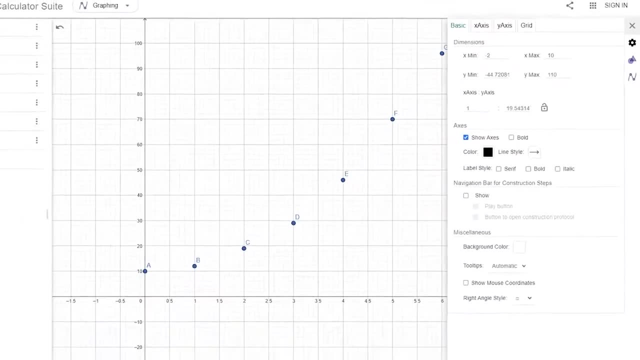 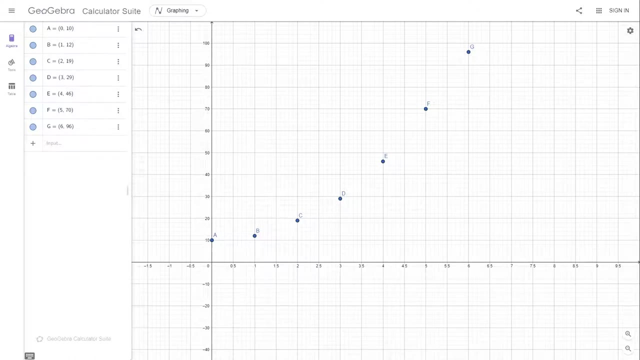 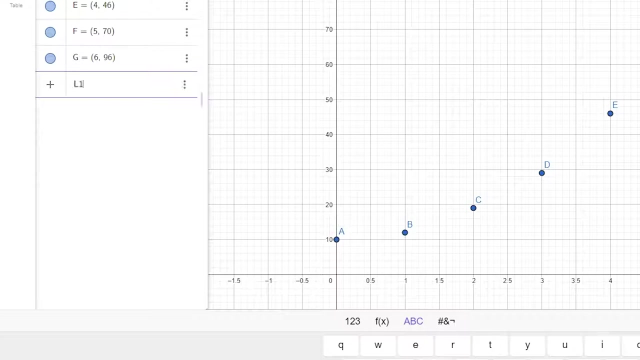 110.. Now we can see all of our data points with an obvious exponential growth curve. Since this data looks like an exponential growth function, we're going to use exponential growth regression. Doing that is simple. First, let's put all of our points in a single list. 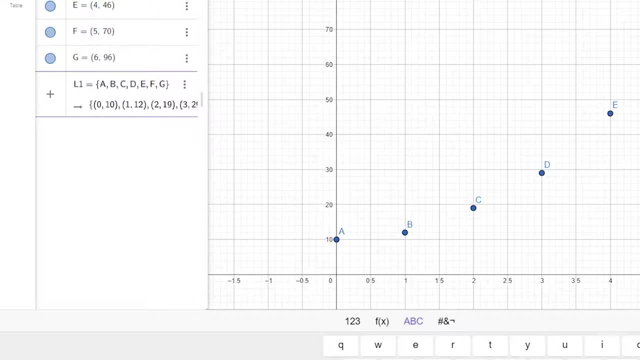 This will make it so that any time we need to use all these points, we only have to tell the calculator what list to use. Now we can see all of our points are in this single list, L1.. The next step is really easy. 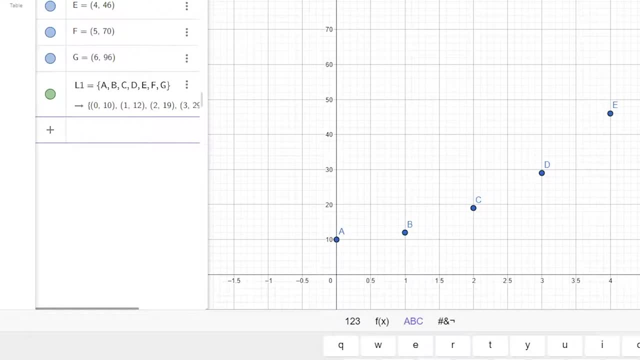 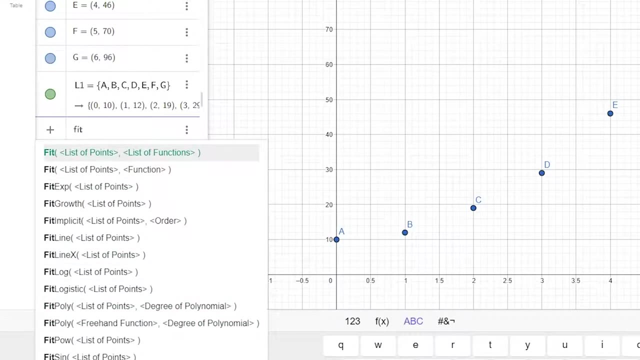 We want to use regression to find the curve of better, So let's type fit. Look at all those different options that pop up. Remember when I said there were different types of regression? GeoGebra is showing us what commands to use for these different types. 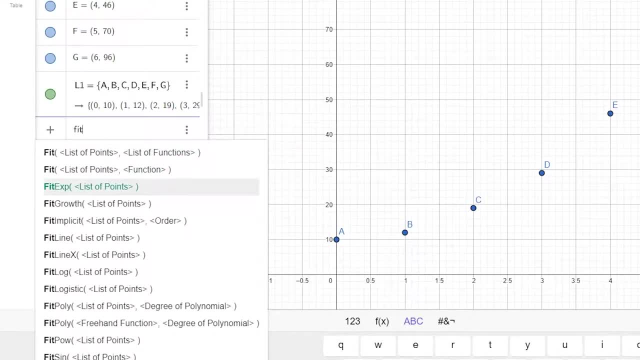 Be careful here. You can see the one called fitexp, but that's not the one we want to use for exponential growth. Instead, we want fitgrowth. Now it wants to know what points to use. We could type the names of all of our points. 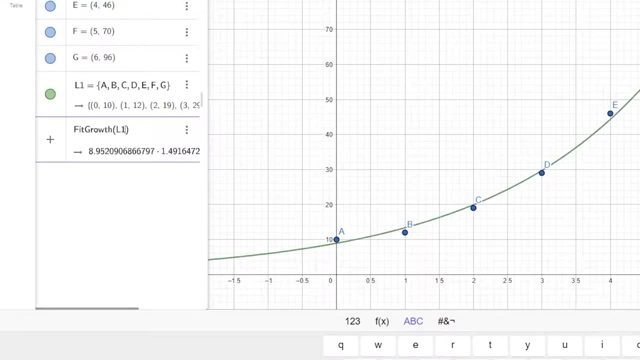 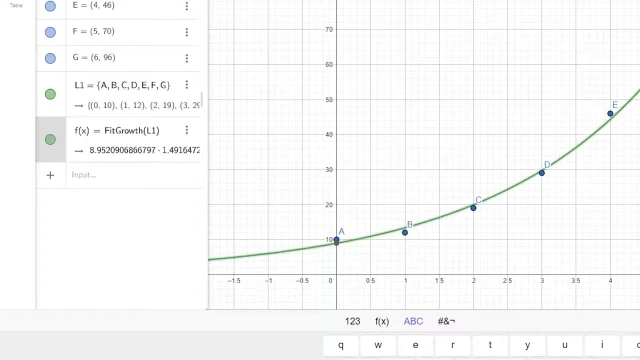 And look, not only did it immediately graph the curve of best fit, it also gave us the equation: The line of best fit is 8.9520906866797 times 1.4916472288649- to the xth power. 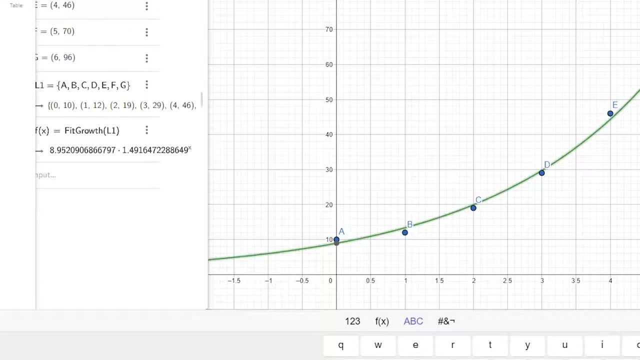 We could round those numbers a little bit, But rounding is general. It's generally a bad idea here As it stands. those are probably irrational numbers that have already been rounded automatically, So we want to keep them as they are instead of rounding any further. 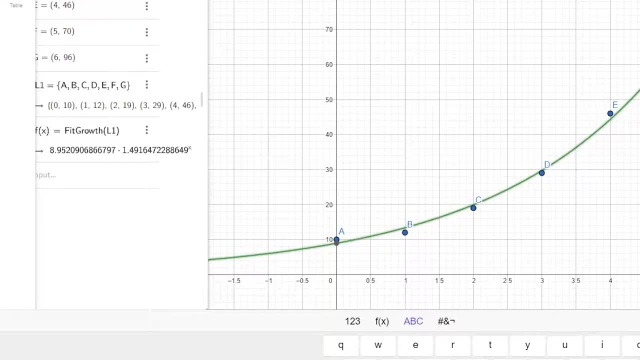 You can actually use the fitgrowth command for both exponential growth and decay, since they have the same basic formula. We can also perform other types of regression. Let's hide the exponential curve for a second and say, hey, that might just be a line. 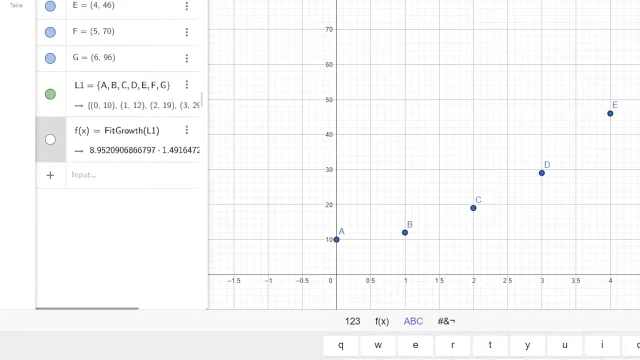 If it is a line, then we're good. If it is a line, then we should use a linear regression on it. instead, Just like before, we'll use the best fit feature, But instead of fitgrowth we're going to choose fitline and give it our L1 list. 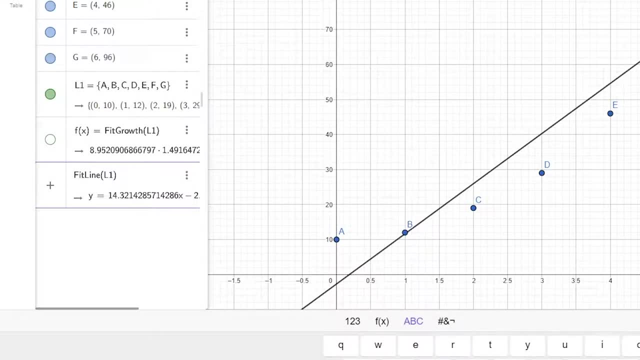 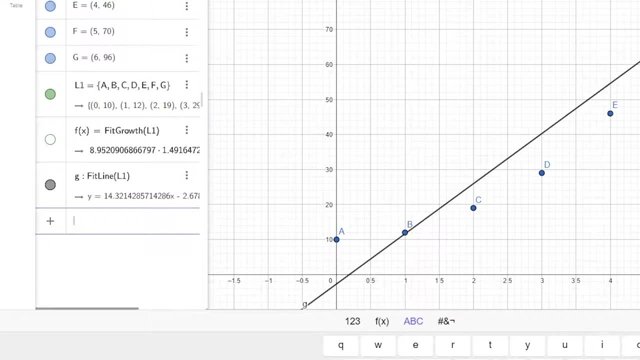 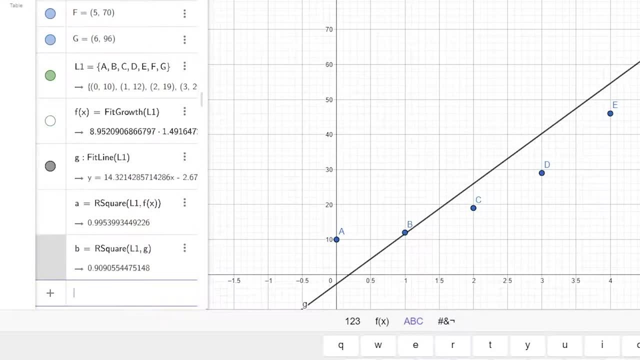 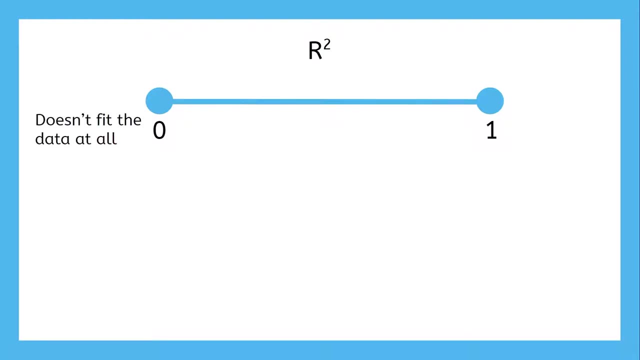 or G. R-squared is a measure of how close to the data the regression is. A zero means that the line occurs or curve doesn't fit the data at all and you shouldn't use that regression, While a 1 means the line or curve fits the data perfectly. In fact, if r squared is 1, that means you didn't. 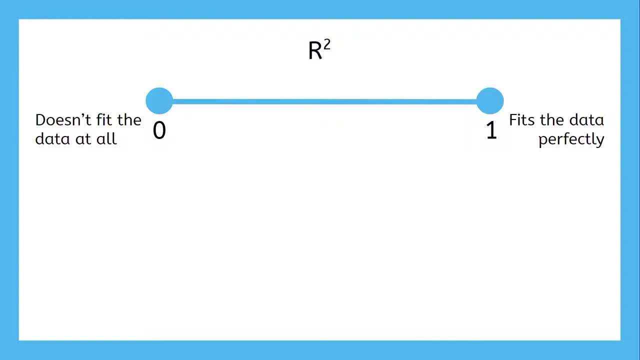 even need regression. You could have found the function yourself. But most r squareds fall somewhere in between. For instance, our exponential growth regression had an r squared value of about 0.9954,, which is really close to 1,, while the linear regression's r squared was at 0.9091,. 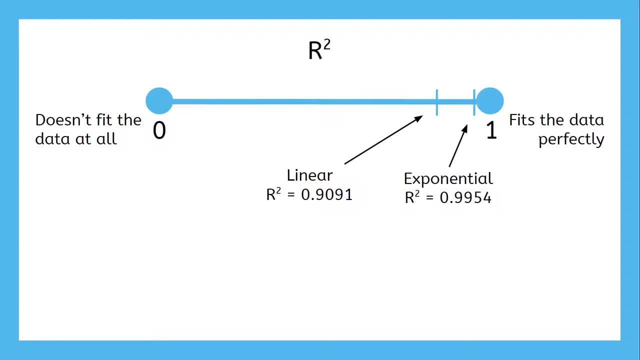 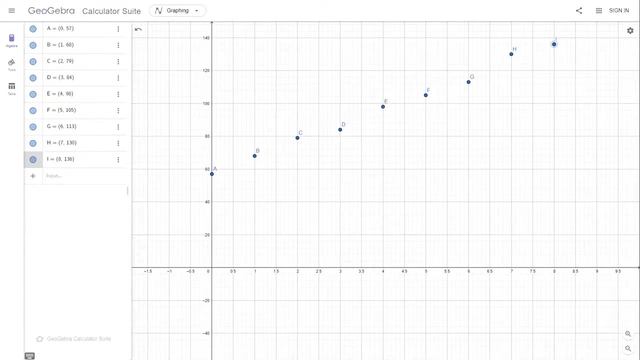 which is a lot lower. What this means is that the exponential growth regression fit the data much better. If we want to approximate this data using a function, we should use the exponential growth regression, not the linear. I've thrown a lot of information at you, so let's put it all to use. Here's a set of data: